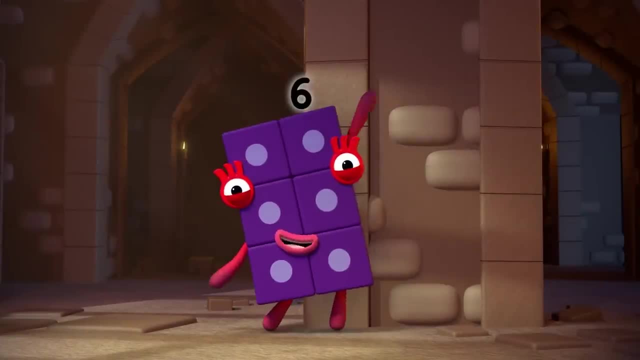 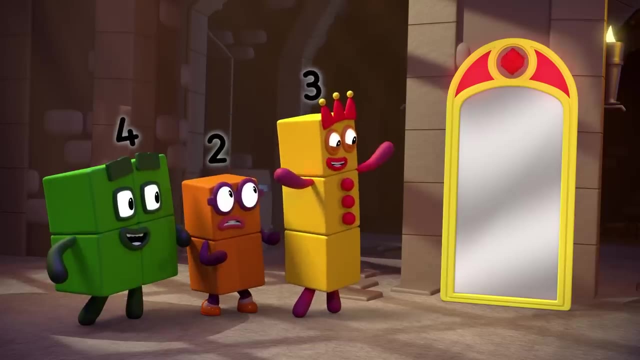 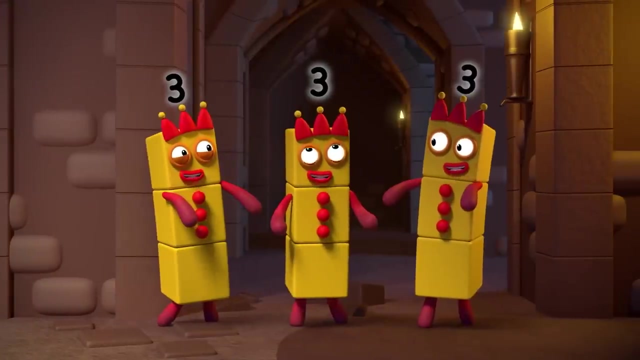 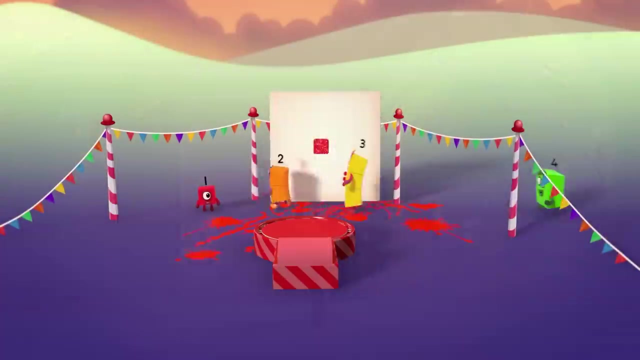 Two lots of three Is six. Number six is on the floor. Don't be shy, Let's have some more Good idea. Three lots, please. Three lots of three Is nine And three, threes, see Yay, Now, now, now You're forgetting something. One, two, three. 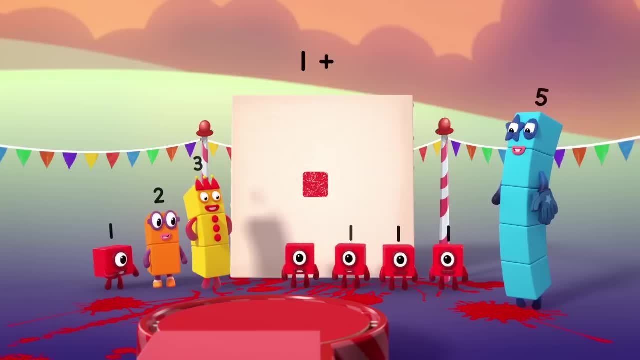 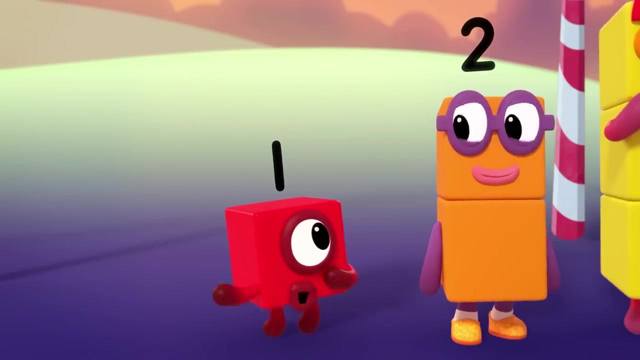 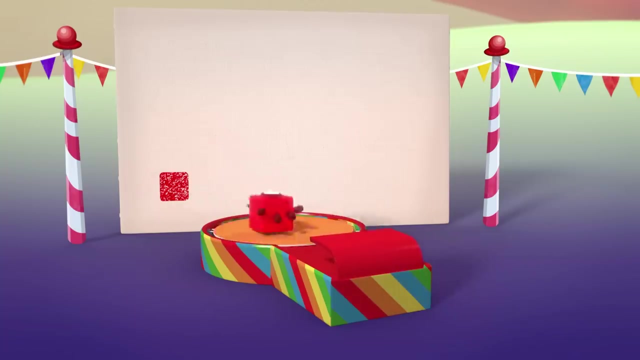 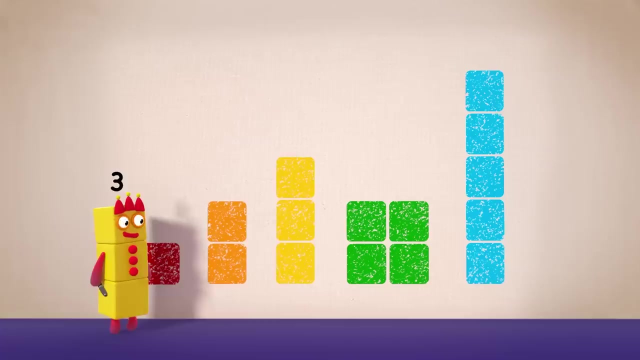 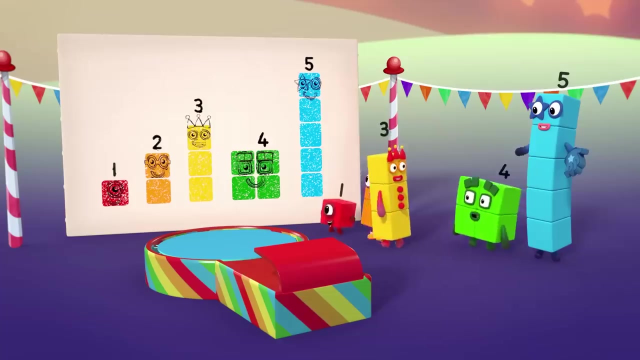 Boo Hey, One plus one plus one plus one equals four. Every big shape is made up of lots of little ones, So lots of little ones can make every big shape. Look what I can do. Yay Ooh, You made all of us All right. 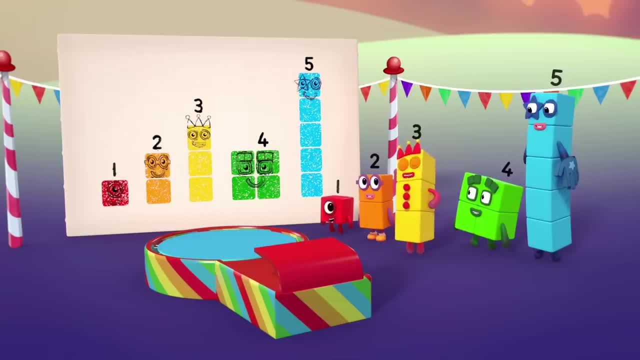 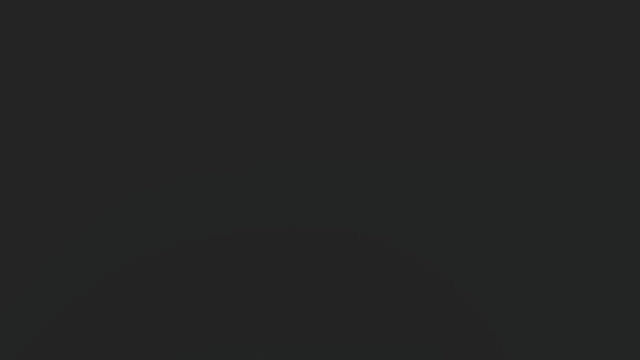 Well done And just in time for the grand finale. What better way to celebrate opening my new park than with fireworks? Ooh, May I present The sky at night? Woo Yay, Woohoo, Yeah, Woohoo, Woohoo. 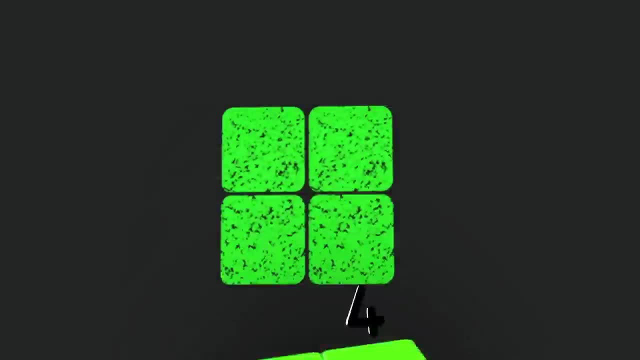 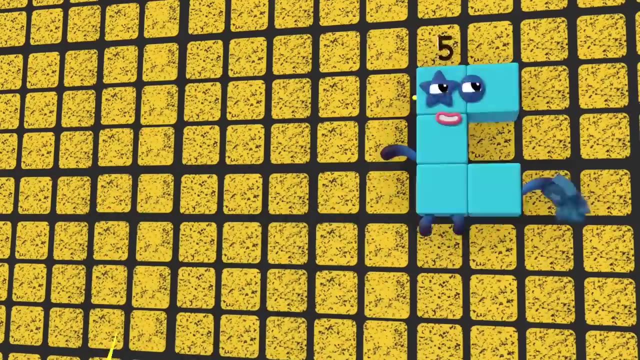 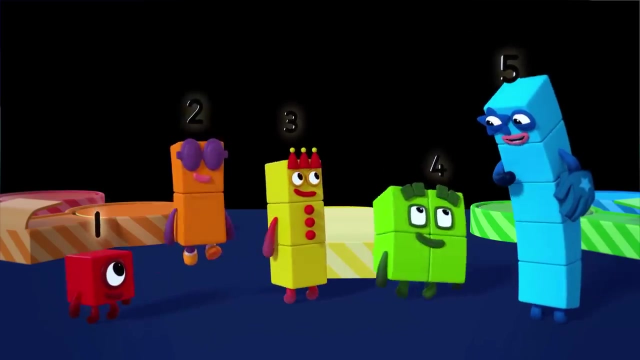 Yay, Yeah, Woohoo, Woohoo, Yeah, Woohoo, Woohoo, Yeah, Woohoo, Woohoo, Yeah, Woohoo. You see one, When we all work together, The sky's the limit. 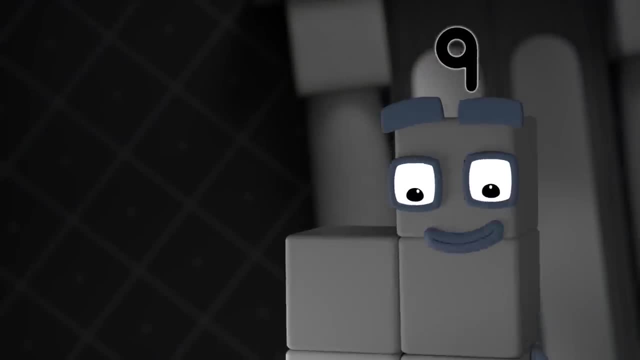 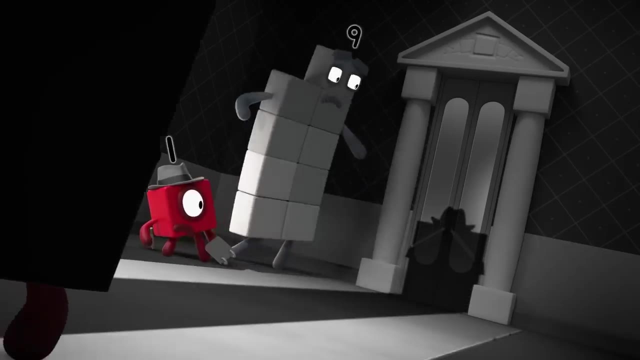 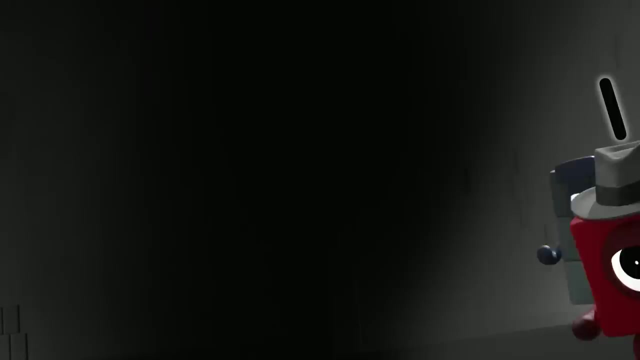 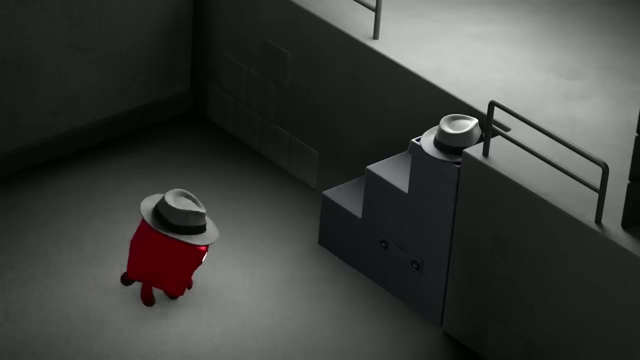 Ooh, Two blocks wide, So they must have been smaller than me. Clue two, Smaller than nine. Look, Hat Coat, It's them. After them, Quick, What Oh There On the steps, The hat Oh. 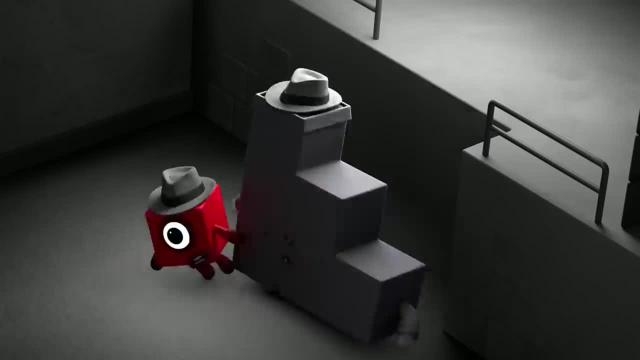 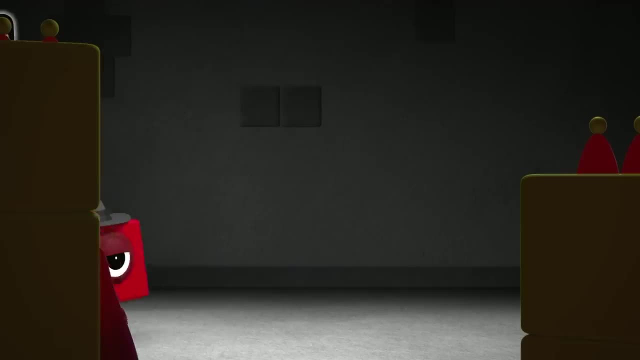 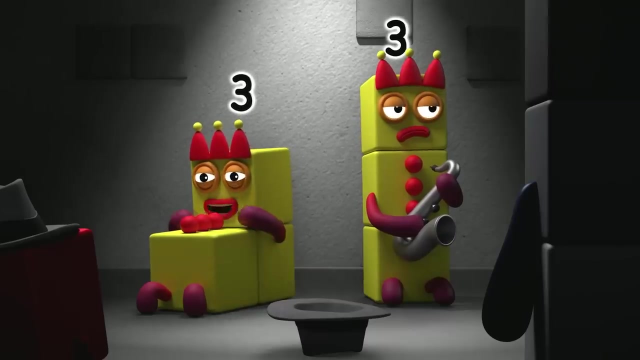 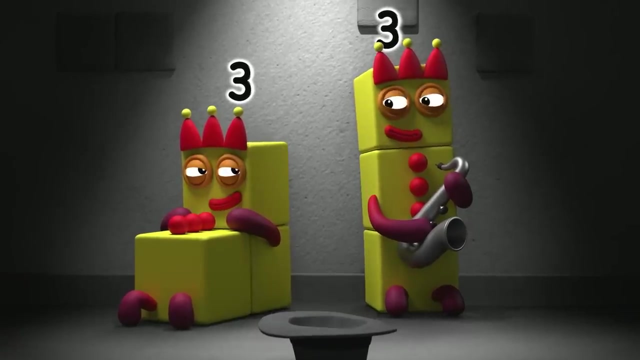 Oh, These aren't steps, It's. Did either of you see a suspicious step-shaped figure in a coat and hat? Sorry, friend, No one else down here, Just us. Something didn't add up, Or did it? Let's look at what we know. 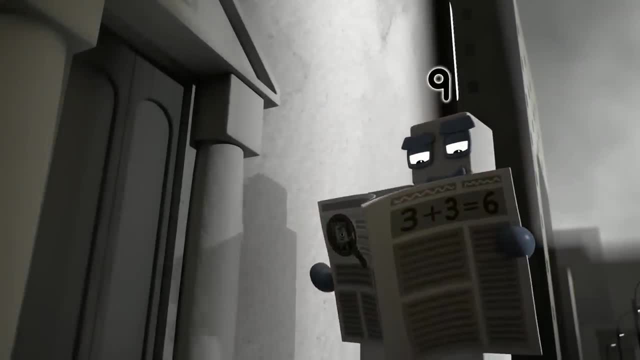 Clue one: The suspect had a flat head when standing two blocks wide, So it can't have been three, five, seven or nine. And it wasn't you, because you can't stand two blocks wide. We need to reach the far side so we can lock the bridge. 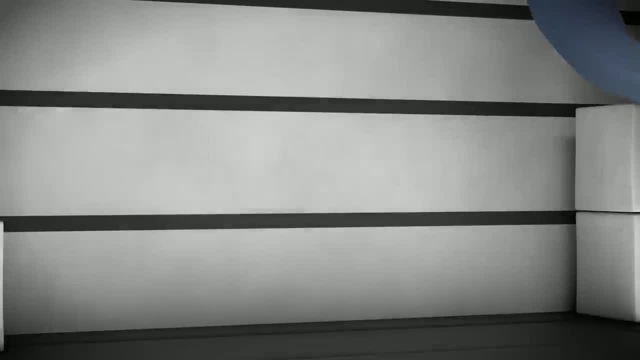 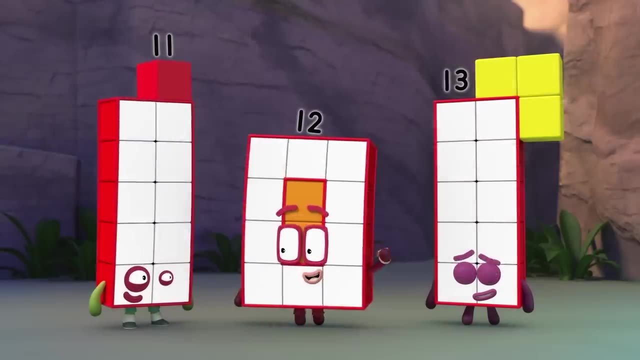 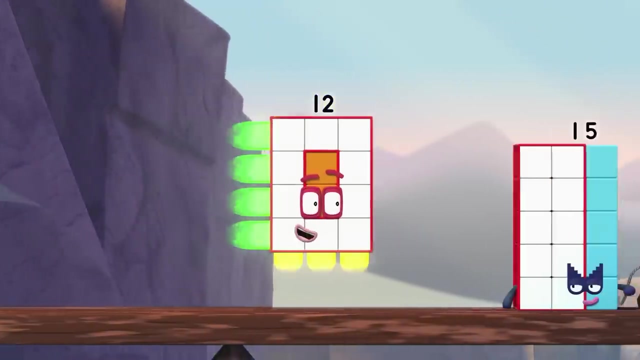 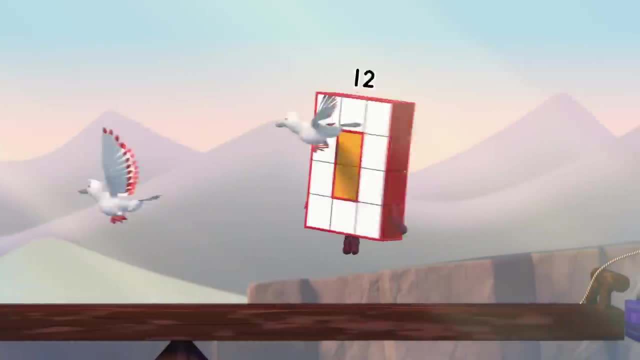 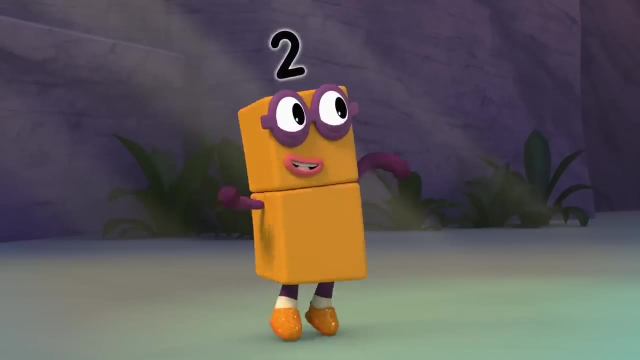 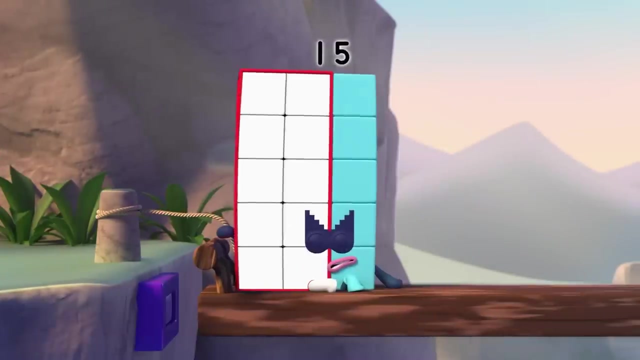 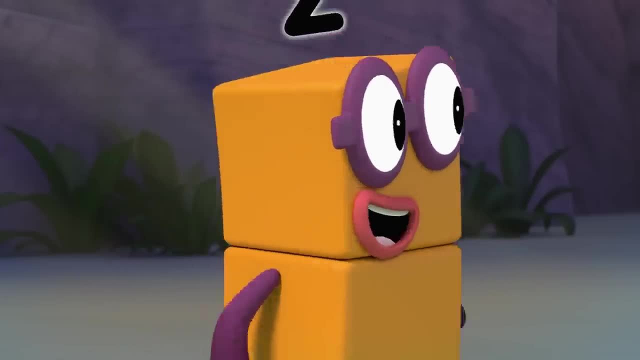 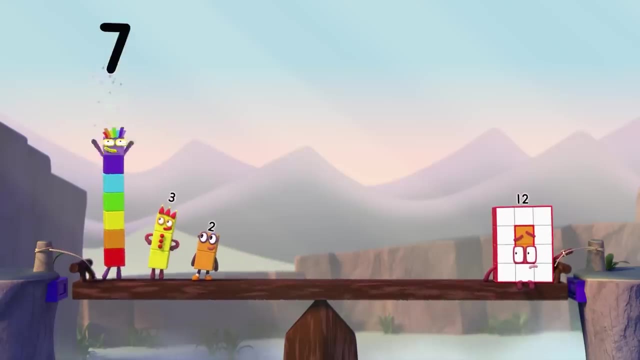 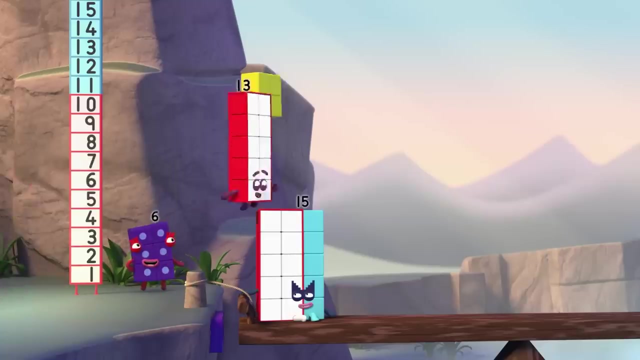 Then we need another ten. Oh, Seven, three, you can make ten. Ooh, That's lucky. Seven plus three Plus two Equals Three. Four Ten plus two equals twelve. Grab hold, Yay, We're halfway there. What could possibly go wrong? 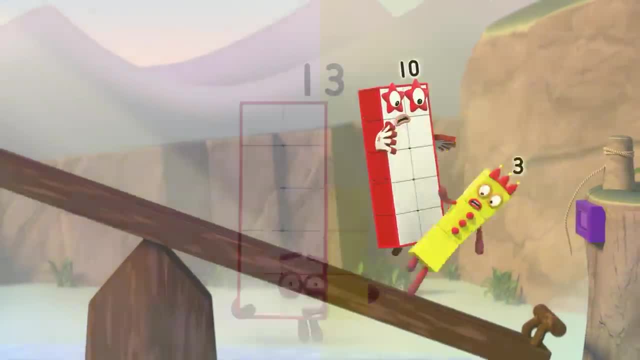 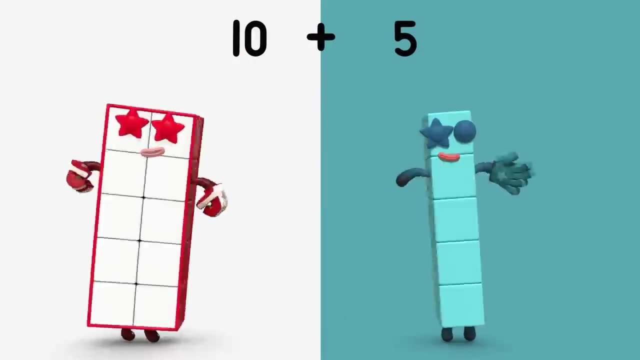 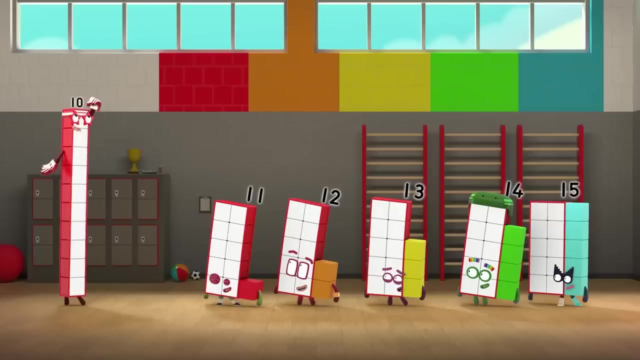 Ooh, Look out 13!. You said it. Oh Huh, Ten plus four is 14.. Ha, Ten plus five is 15.. Terrific, Now let's stretch our tens nice and tall. Fling those ones high in the air. 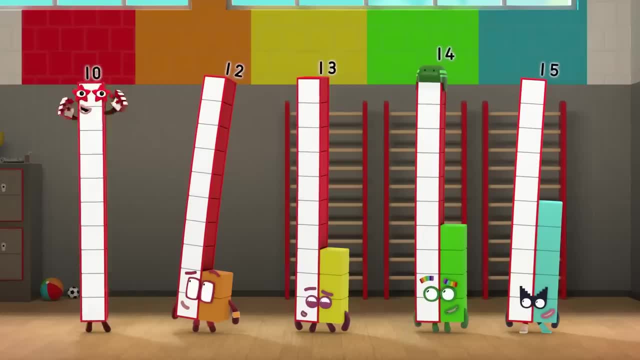 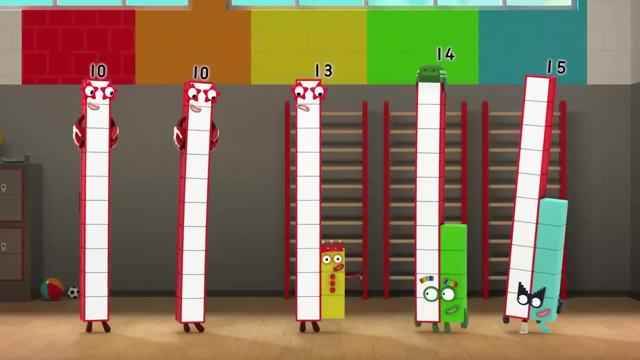 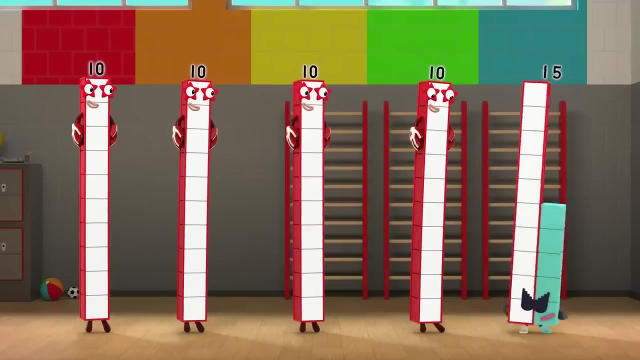 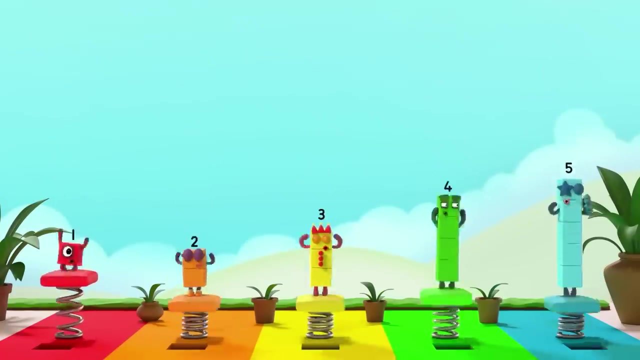 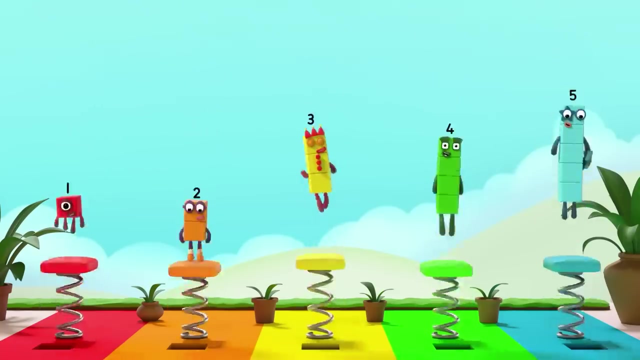 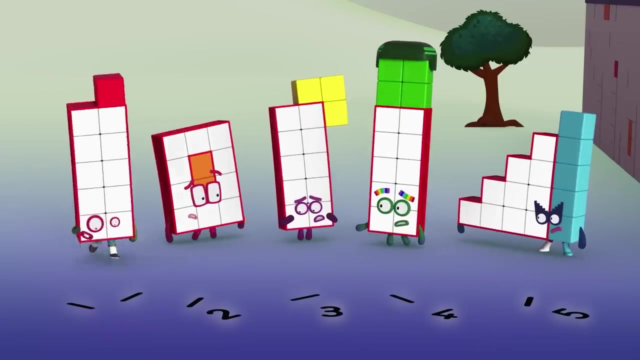 Take it away: Eleven minus one is ten. Twelve minus two is ten. Thirteen minus three is ten. Fourteen minus four is ten. Fifteen minus five is ten. One minus six is twelve. One, Two, Three, four, five. 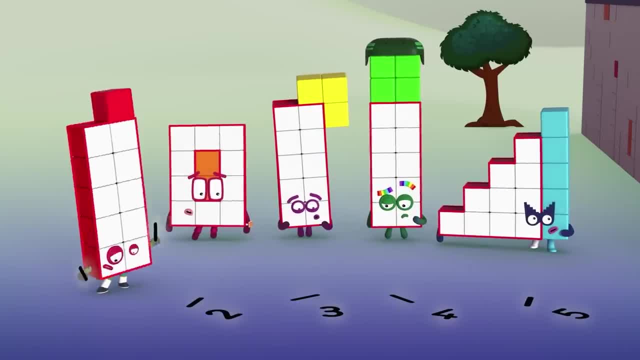 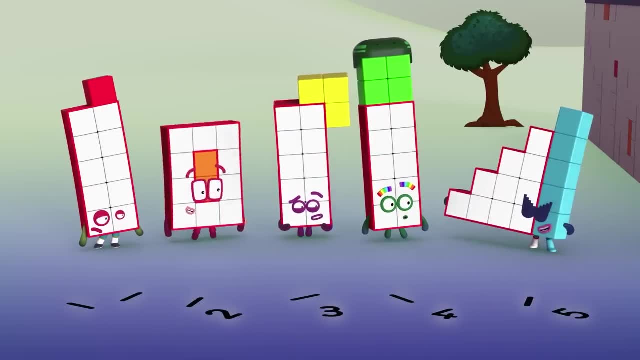 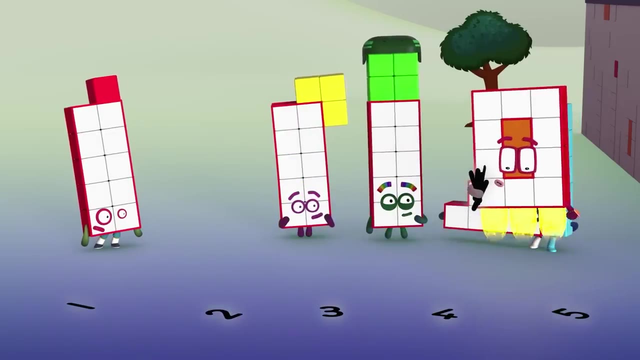 Numberlings A… Boy, WOO, We've all got more than one block. I've got one, Um, well, more than one anyway. Arranging things neatly in rows can help. Let's put all the wands here. 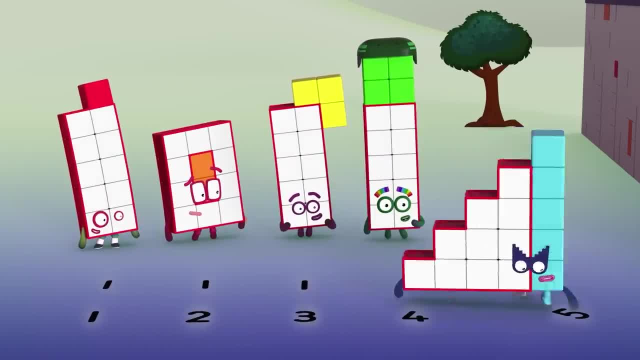 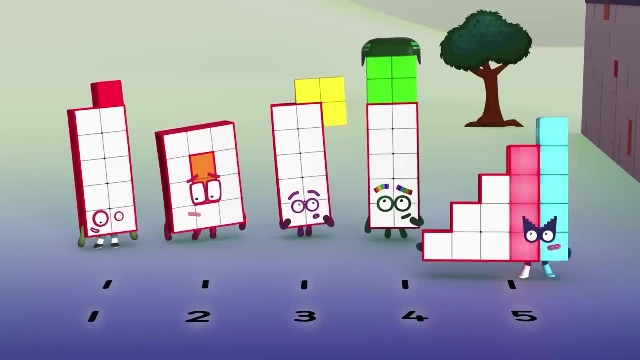 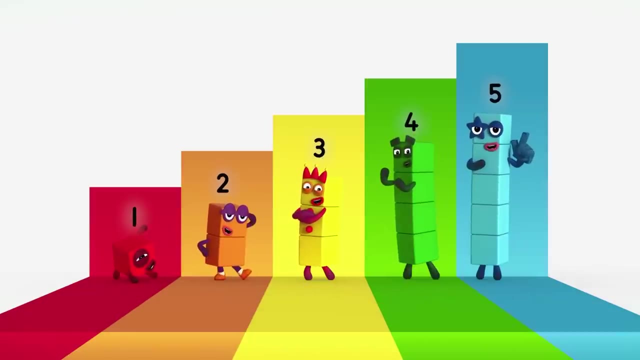 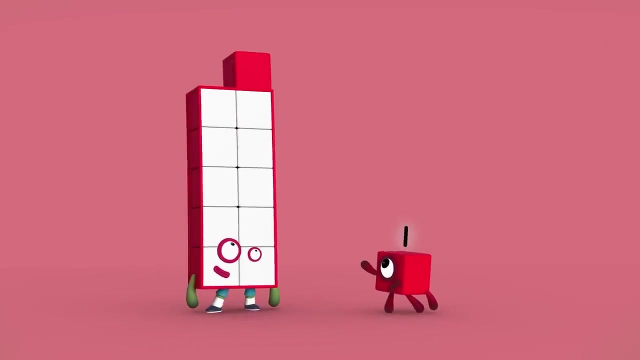 And then this feels right: One, two, three, four, five. Hmm, that feels familiar. One, two, three, four, five. Hush, hush. The super special secret step squad is here. Step one: Look on top of your big block. you've got one red block, like me. 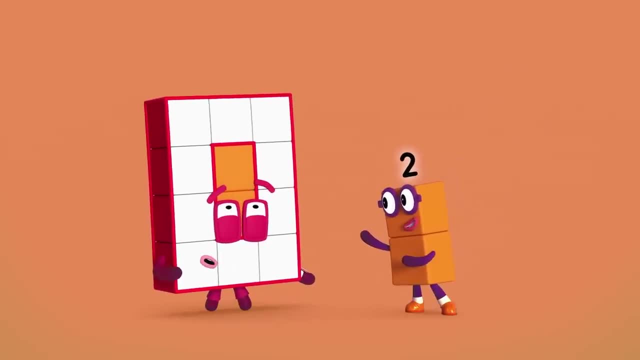 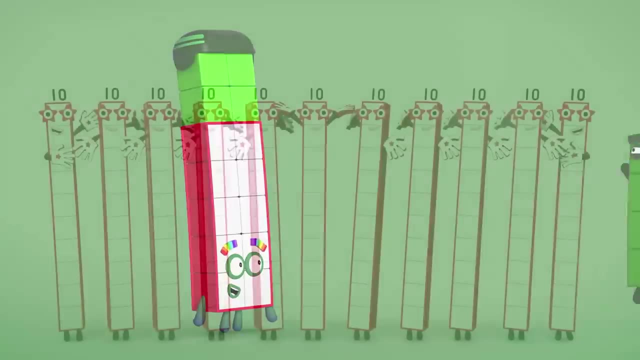 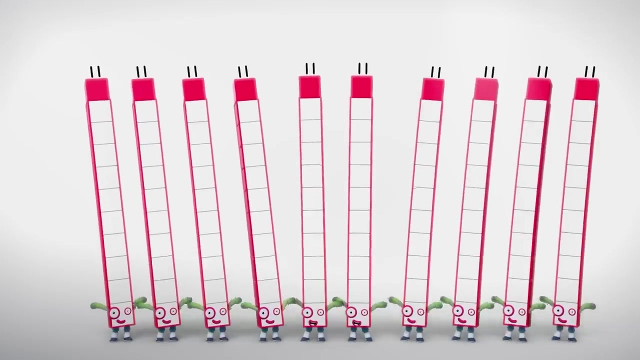 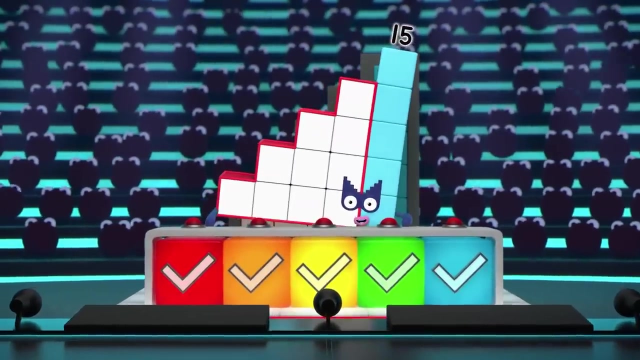 Step two: You've got two orange blocks, like you. Step three: Look at me. Ho, ho, ho, ho, ho. Step No, Brick-a-dab-bra. Step eleven: Now it's time to see what some of our bigger numbers have in store. 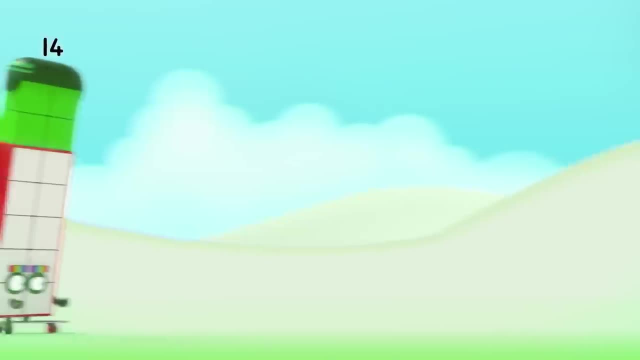 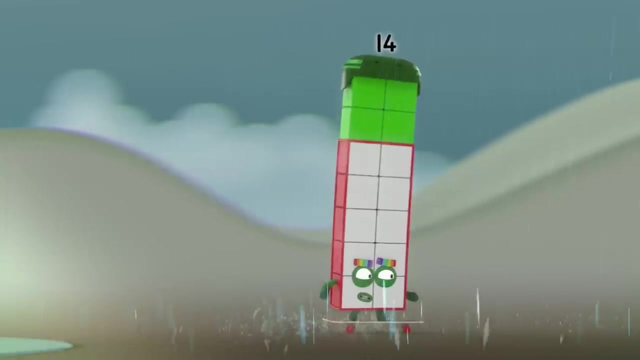 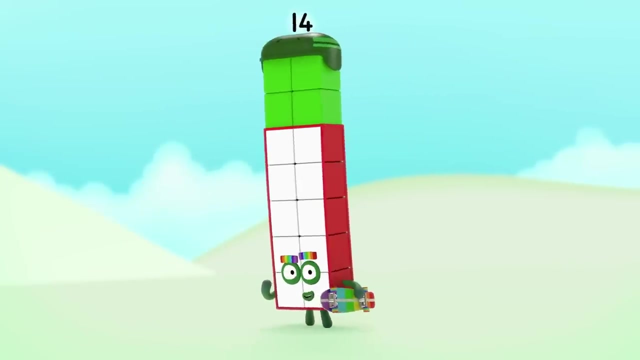 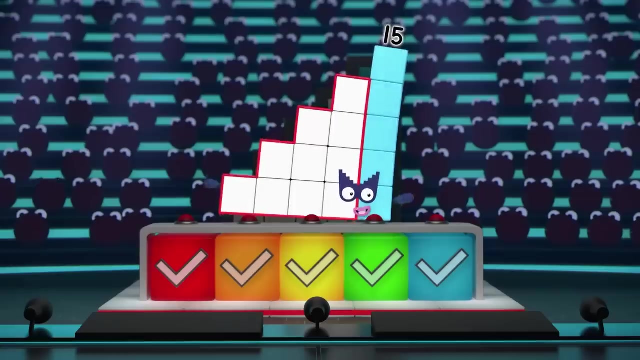 For as long as I can remember, I've always wanted to skate In wind, Rain And snow, No matter how gnarly it gets. I put in the hours Because practice makes perfect. Welcome to Fifteen's Minute of Fame. 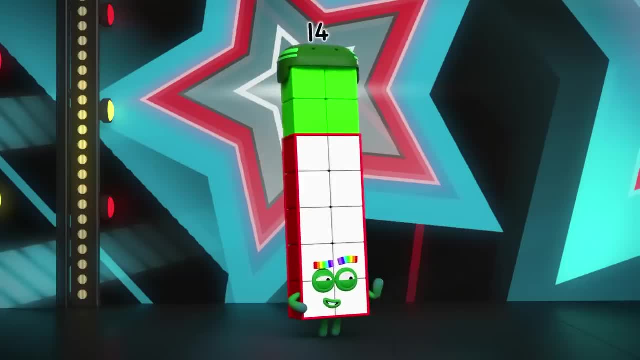 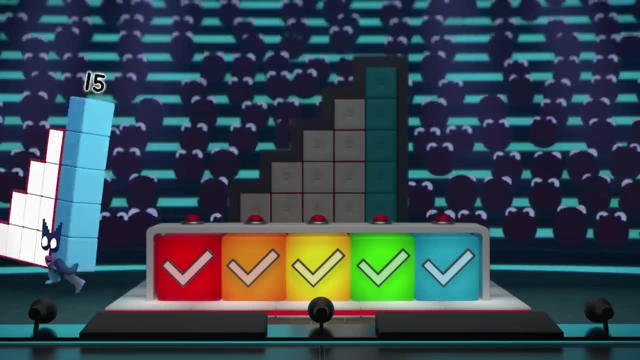 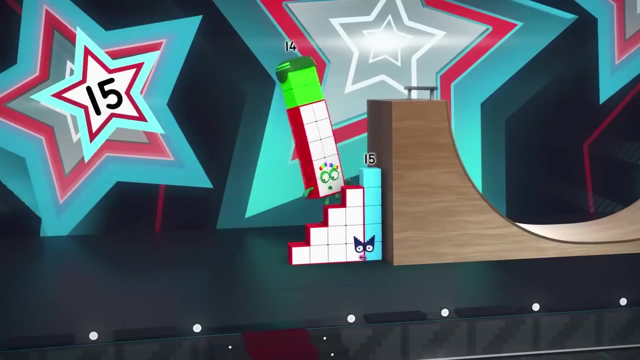 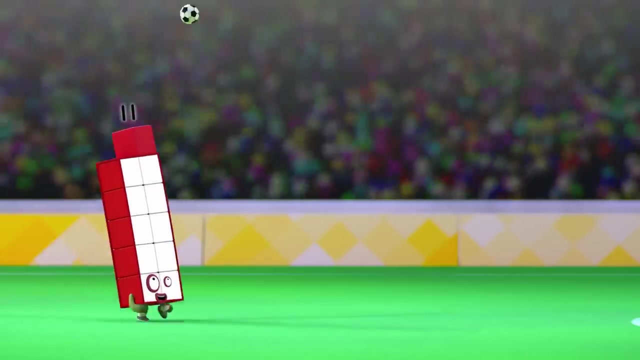 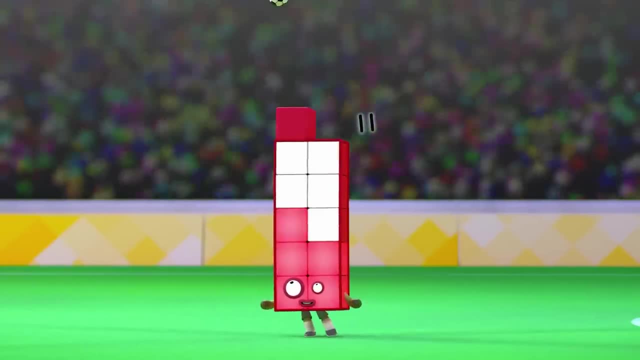 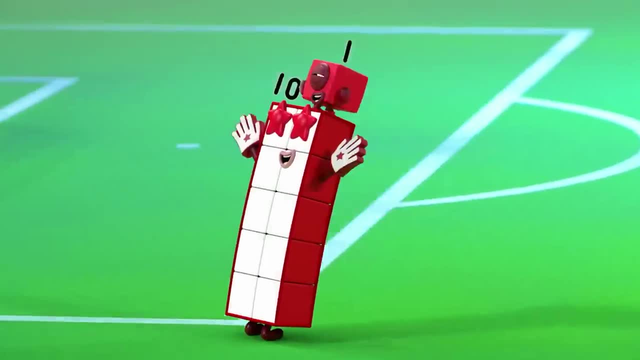 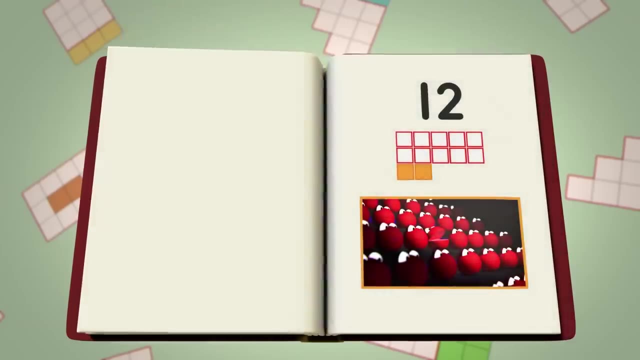 And one more. He's eleven, She's six, She scores One ten, One, one. There's only one. eleven, Chapter twelve: Rectangle rush: Yay, Hooray, Yay, Hooray, Hooray. 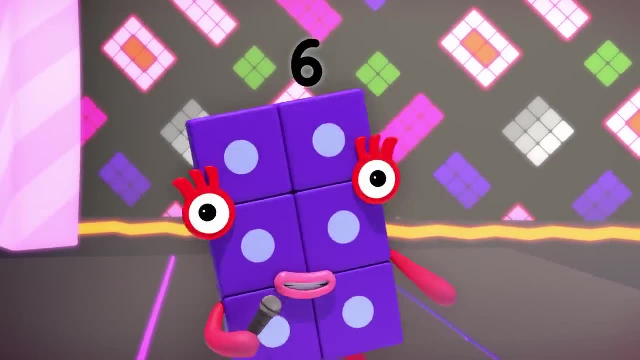 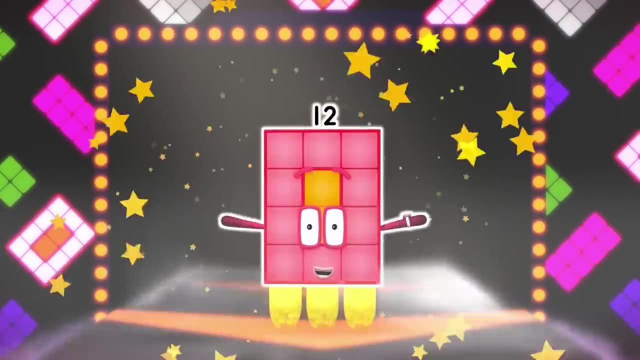 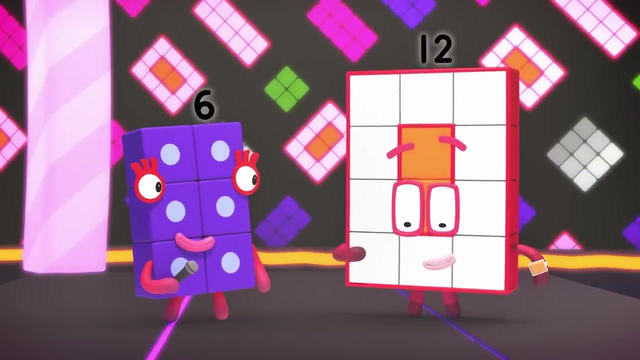 Yay, Yay. Welcome to Rectangle Rush. Let's see who's next to brave the crush. I am 12 and I am a super rectangle. That means I can make lots of different rectangles. Show us what you've got. Game on. 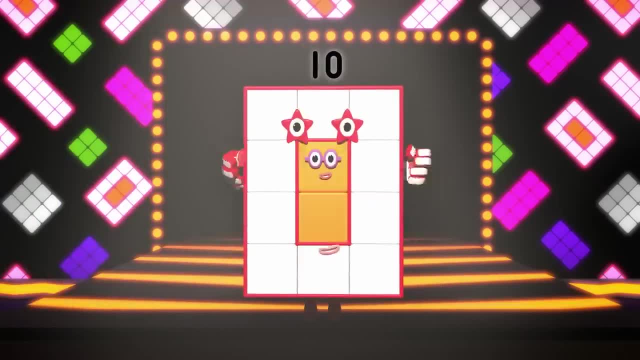 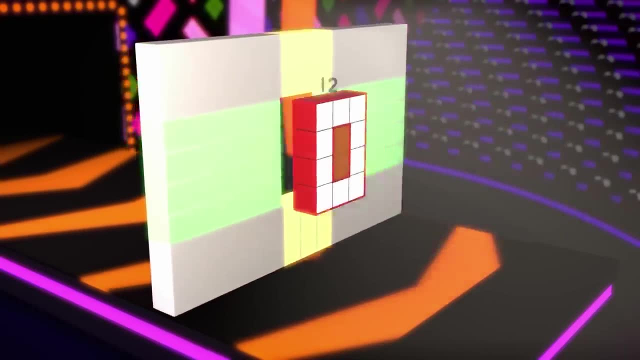 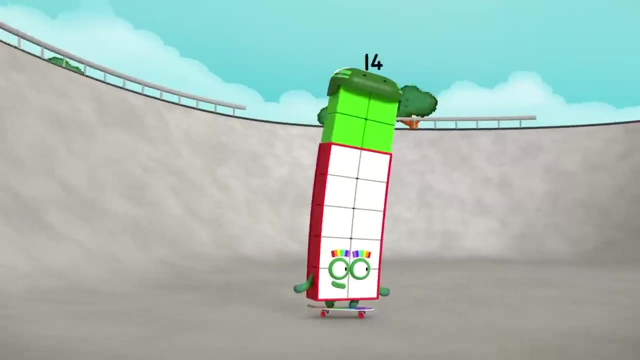 I am 12.. I am 10 and 2. And I am 3 blocks by 4 blocks. I am a Sooner or later I'm going to be a skater. I'm 14.. I'm 10 and 4.. I'm also double 7.. 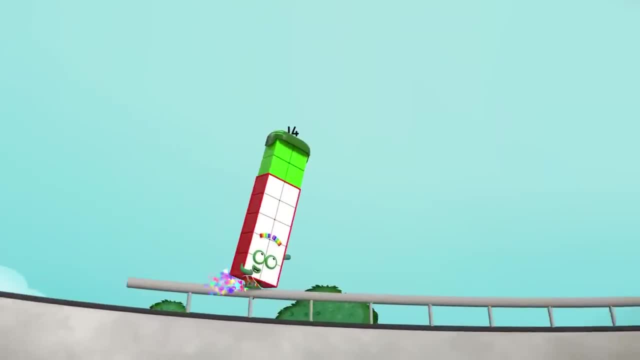 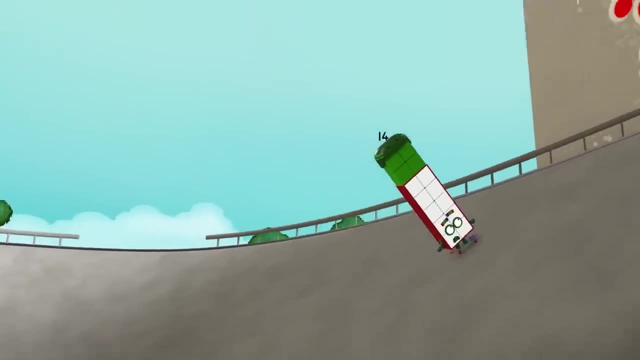 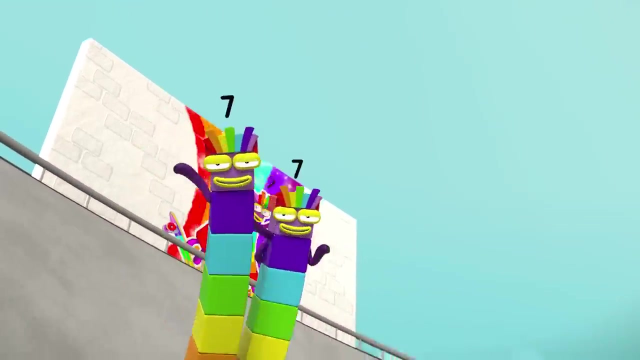 I'm riding on an elevator straight to skater heaven And whenever I get into a fix in the middle of one of my brand new tricks, I've got my lucky double to get me out of trouble. Lucky double 7.. Maybe you've got a lucky double too. 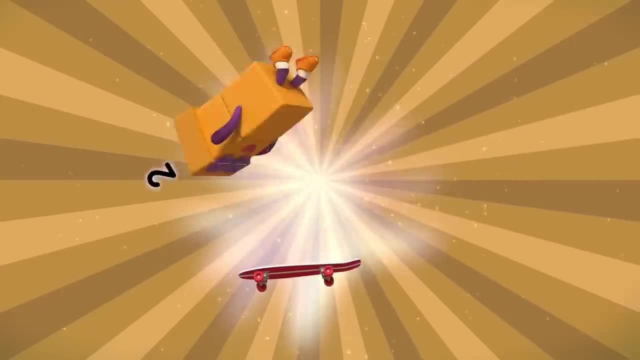 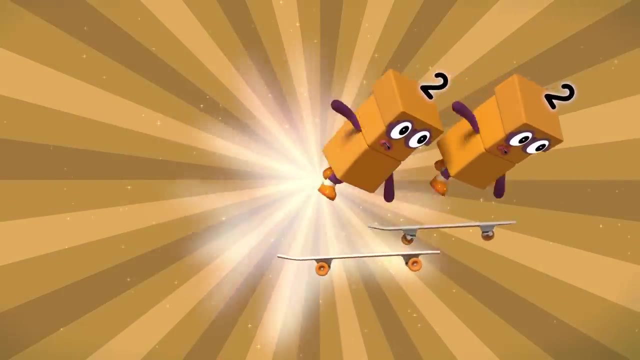 Hello, I'm 2 and I can split into ones Double 1, double the fun. I'm 4 and I'm double 2.. Whoa, two, twos. I think we may need grippy shoes. I'm 6 and I'm double 3.. 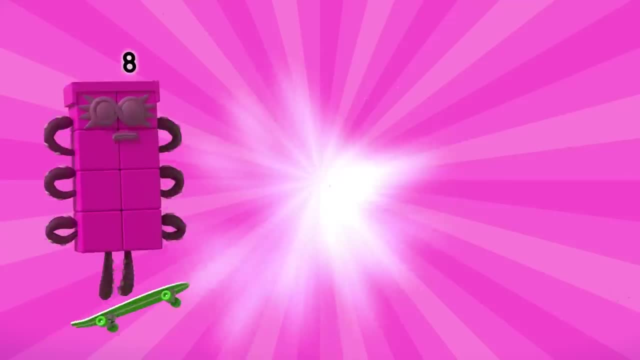 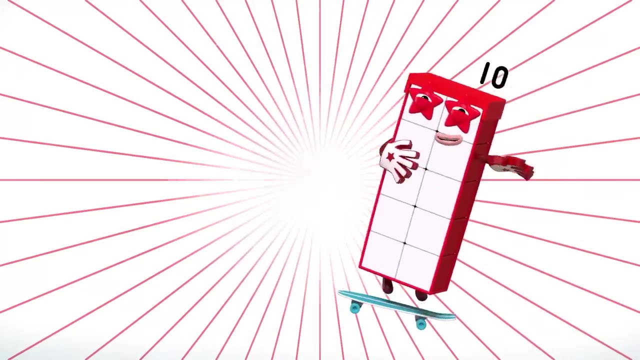 Well, we'll be saying: look at me, I'm 8 and I'm a 4 and a 4. Double 4.. Have you seen us before? I'm 10 and I'm double 5. Two big hands. Now we can do a double 5 hand jive. 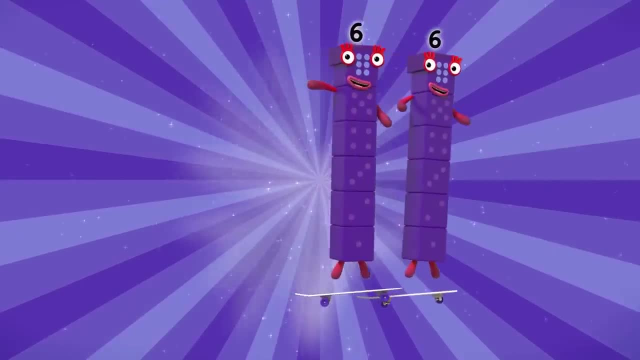 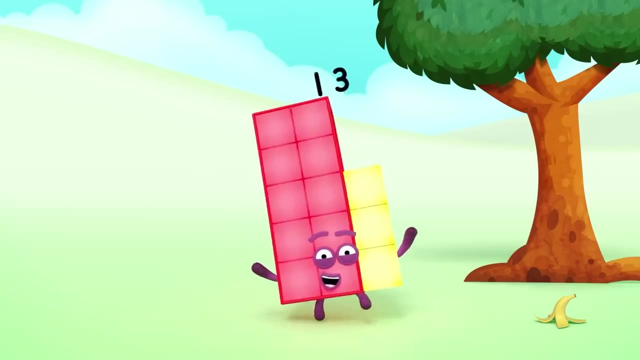 I'm 12 and I'm double 6.. We don't need dice to do these tricks. I'm 1, 2,, 3,, 4,, 5,, 6,, 7,, 8,, 9,, 10,, 11,, 12,, 13.. 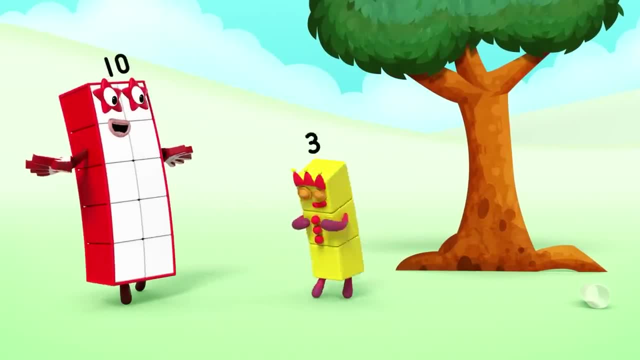 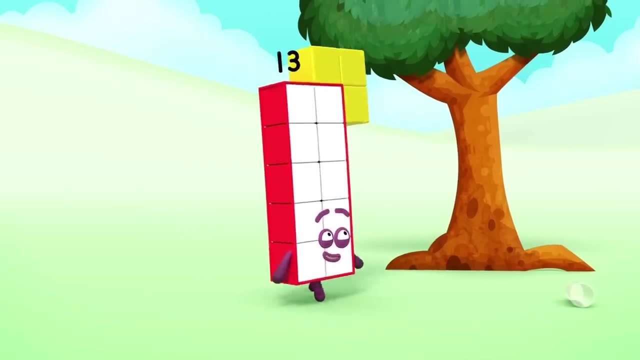 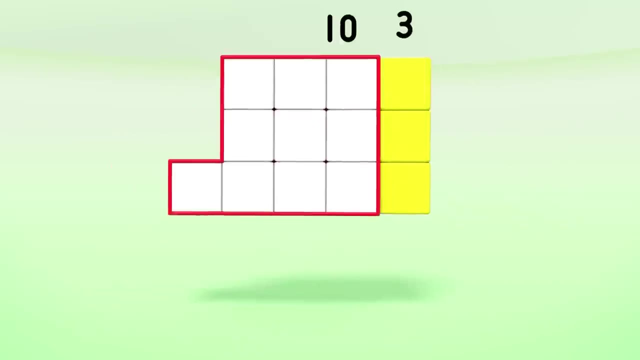 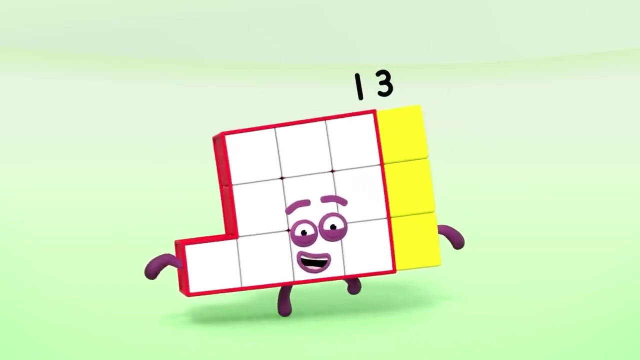 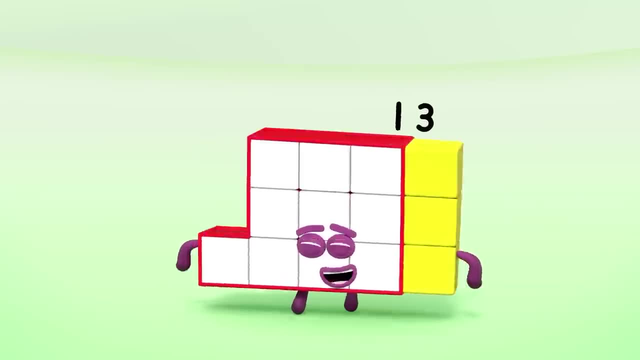 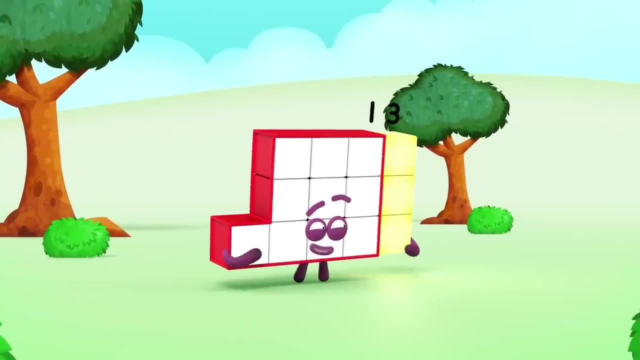 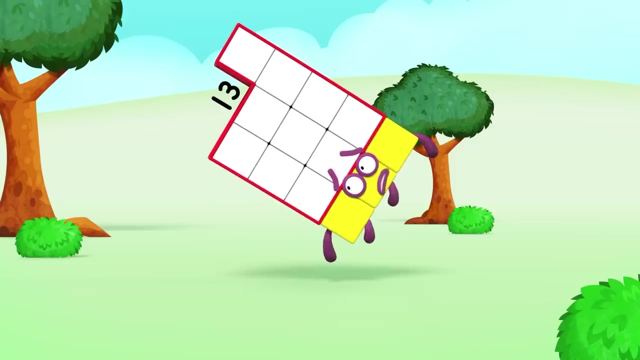 Hooray, Hooray, Hooray, Hooray, Hooray, And I think I might be a little bit unlucky. This is me, 10 and 3, expecting to run out of luck. Sorry, It's all jolly japes when I get into scrapes. 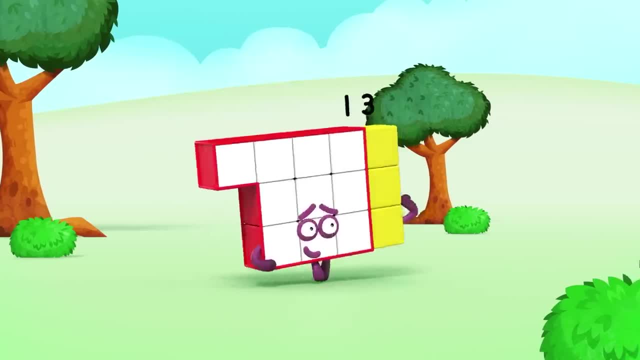 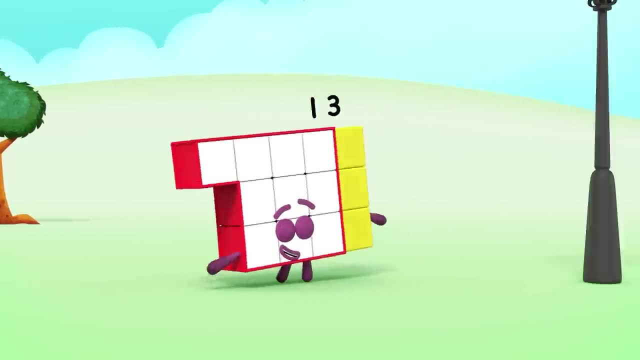 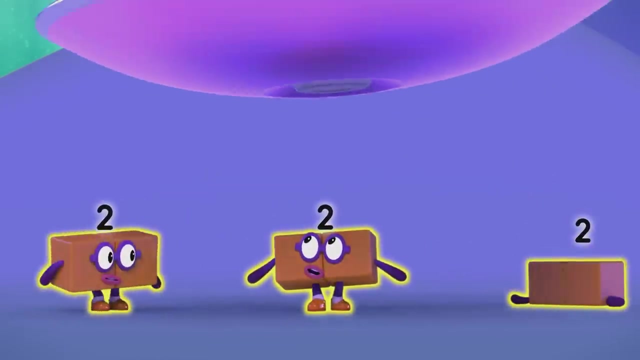 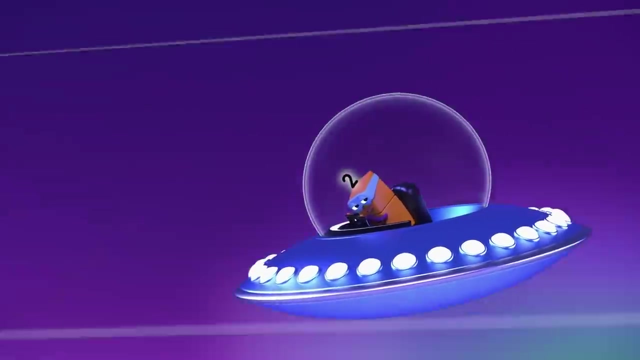 I'm always coming unstuck. I'm the clumsiest number you've ever seen. Unlucky, Unlucky Number 13.. It happened again. A three Happy, Terrible Tuesday, everyone, Or should that be every two? 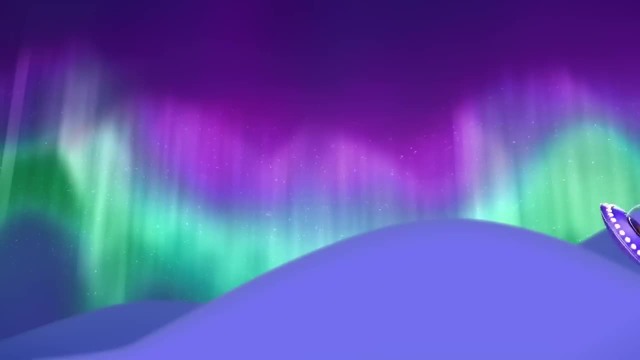 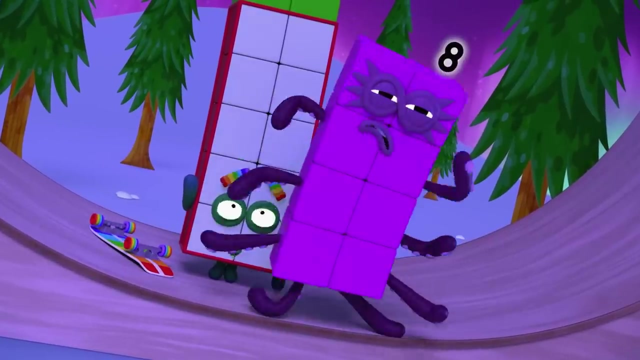 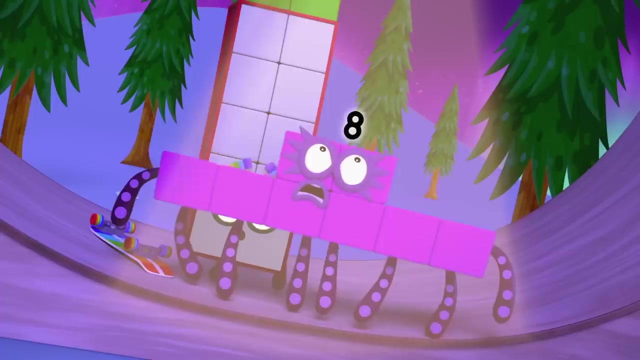 Target acquired, Never fear 14.. I've dealt with the terrible twos before Off to block shield. One, two, three, four, five, six, seven, eight, Eight, One, Hey, Two, Hooray. 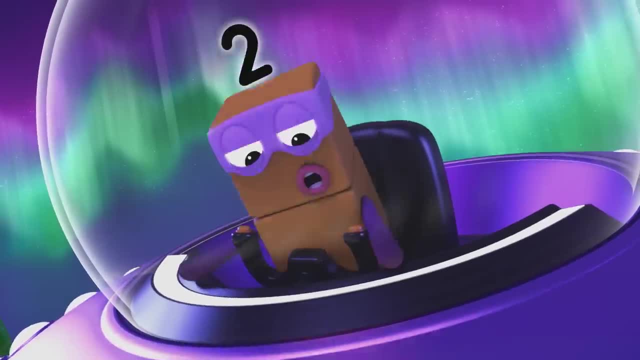 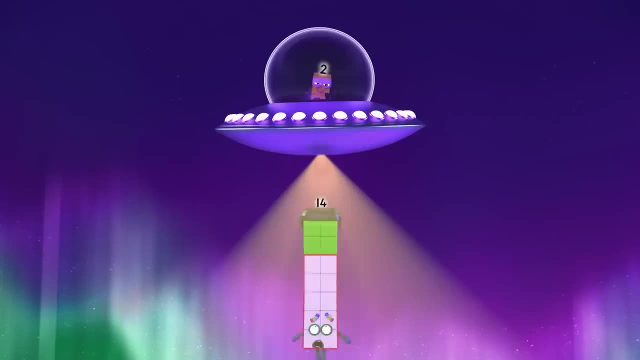 Three, Hey, Four, Hooray, There are four twos in eight. You're in the lead, amigo, but not for long. Woo-hoo. One, two, three, four, five, six, seven, Oh pretty. 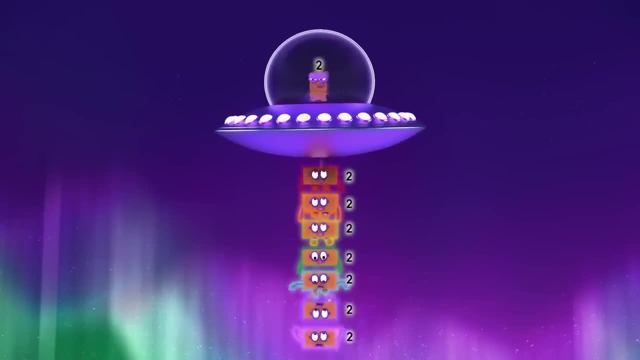 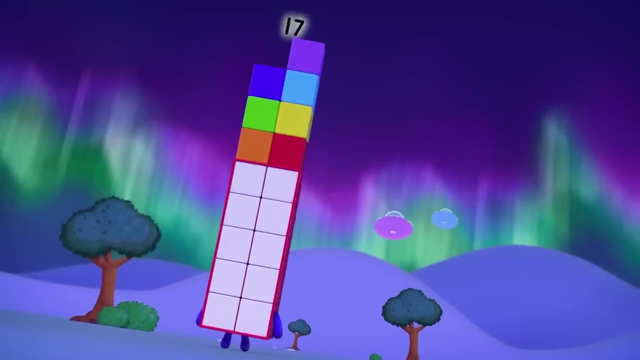 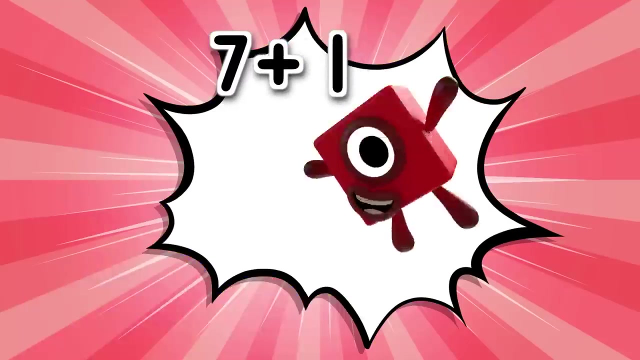 There are seven twos in 14.. Beat that, Excuse me, I need to lend a hand. Hold still, Seven Was Seven. Was One Equals Eight. Octoblock leap One, two, three, four, five, six, seven, eight. 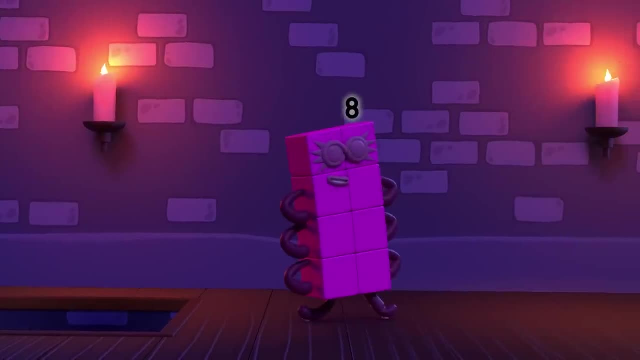 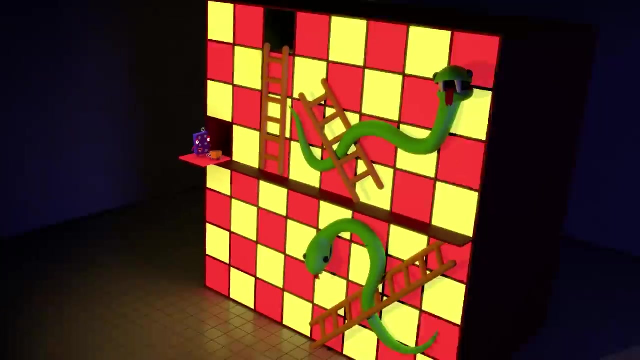 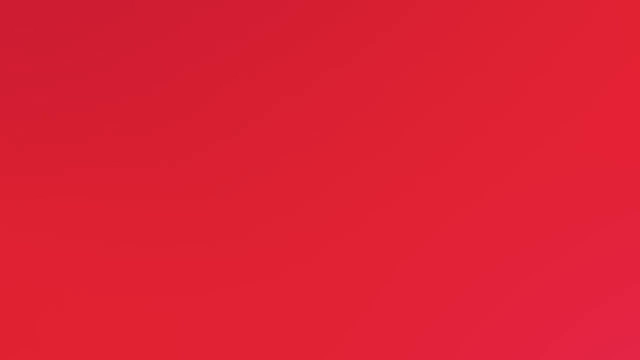 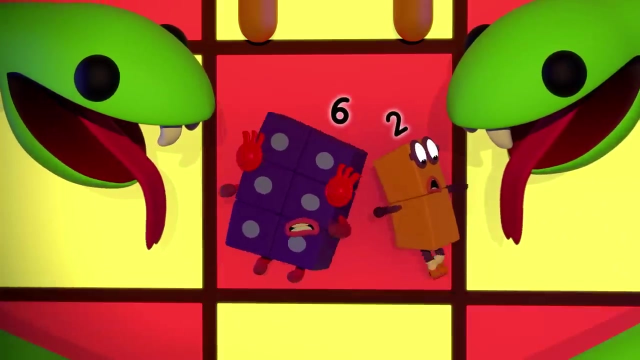 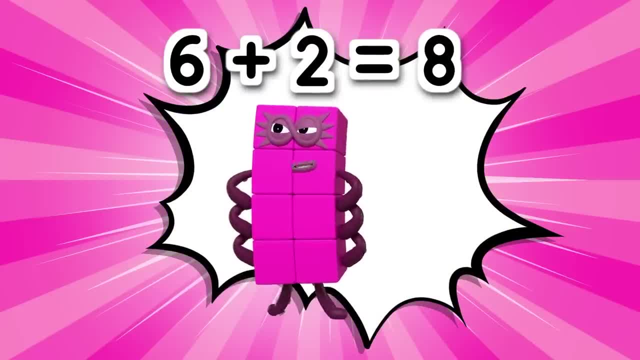 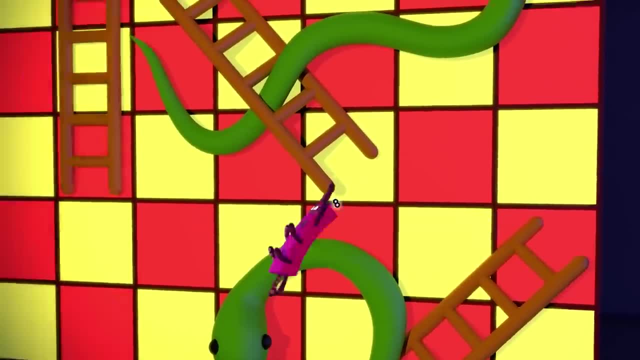 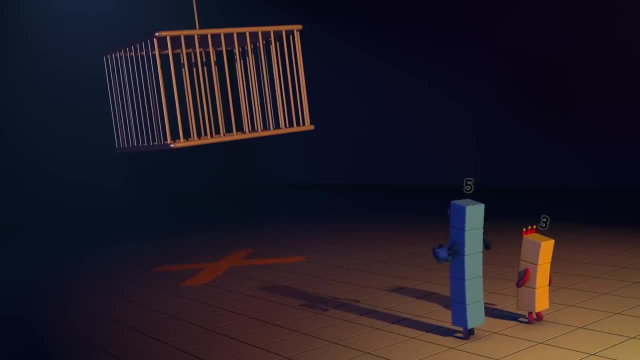 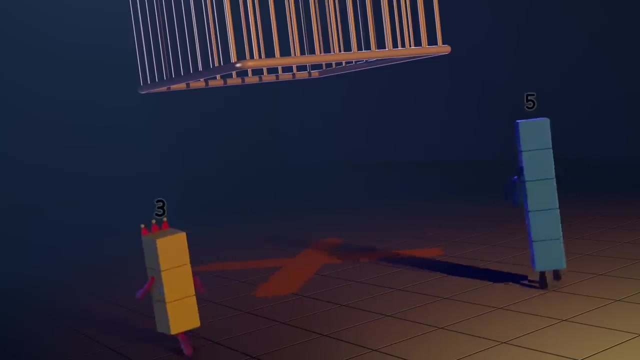 Six plus two equals eight Octoblock climb. One, two, three, four, five, six, seven, eight climb. Uh, They won't catch us that easily. Don't walk under the cage. I could just Resist it. 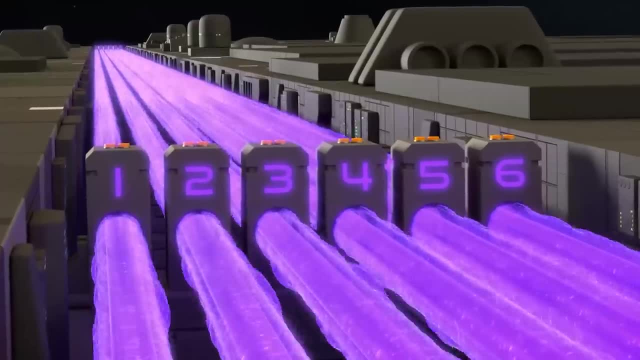 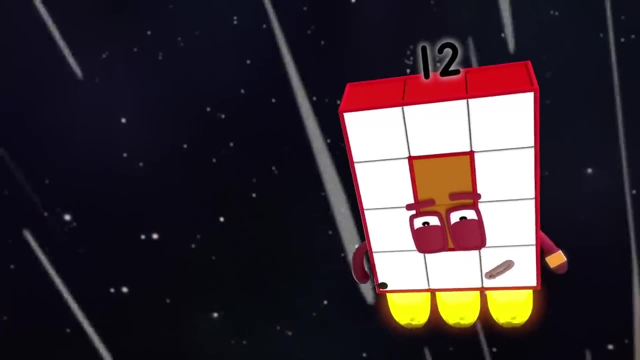 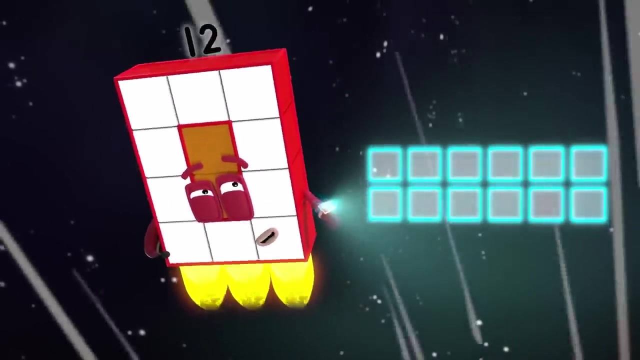 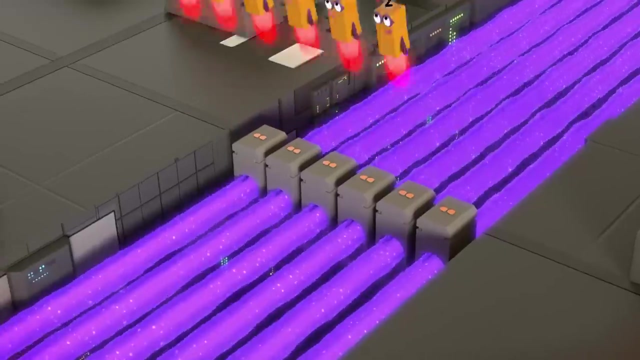 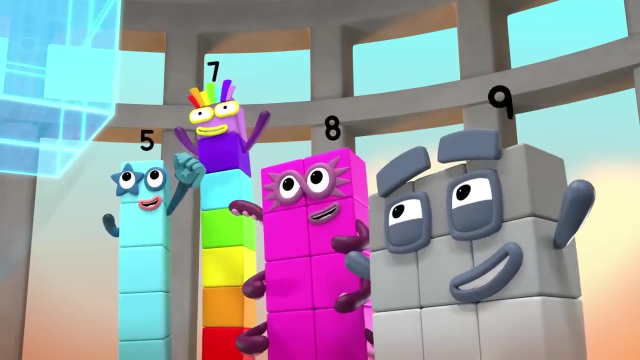 Can you see a line of towers ahead? Yes, six of them. Each has two buttons on top. You need to press all the buttons together. Six towers, two buttons each Array display. This calls for switch Wee Six teams. Whoa Lucky. 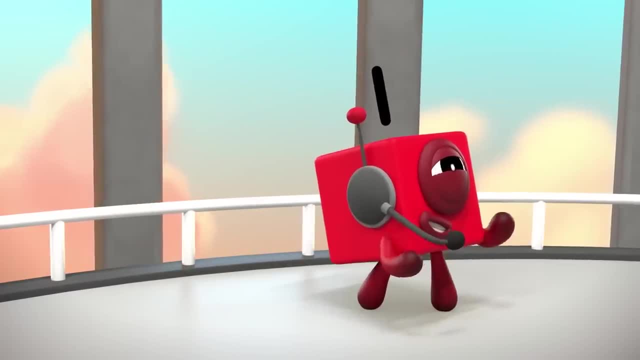 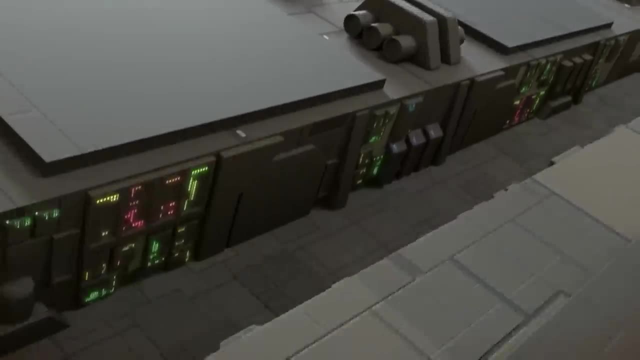 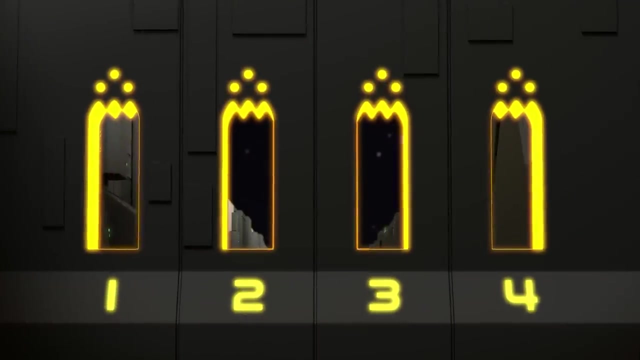 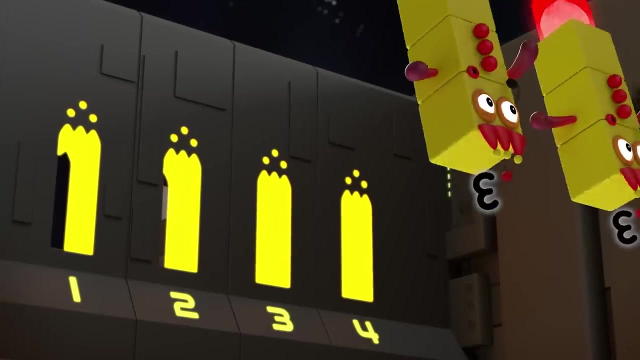 You've done it. Twelve. Now head for that battery. There's no time to lose. I'm on it. Switch, Pull up Twelve. You're going to hit. No time. Turn For a breeze. How do we ride them? 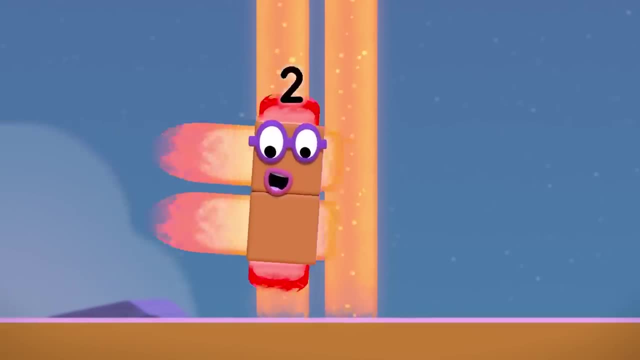 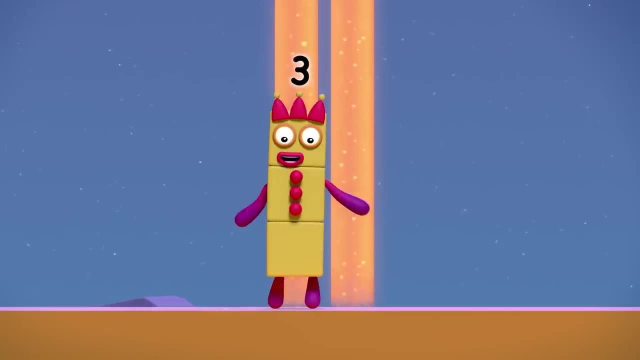 These are two rays, So maybe Wee Come up. It's fun. Oh, that's no use. I can't make a rectangle that's two blocks wide. No, But I can. I'm a two by two square- Wee. 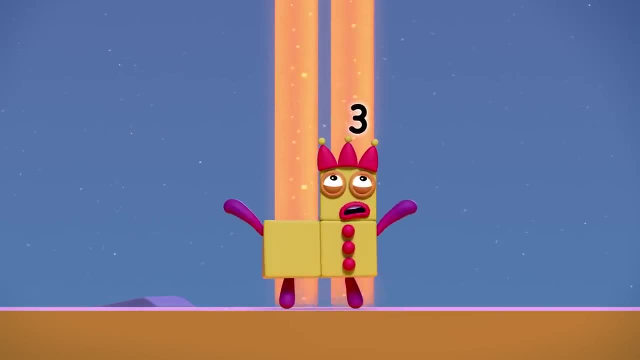 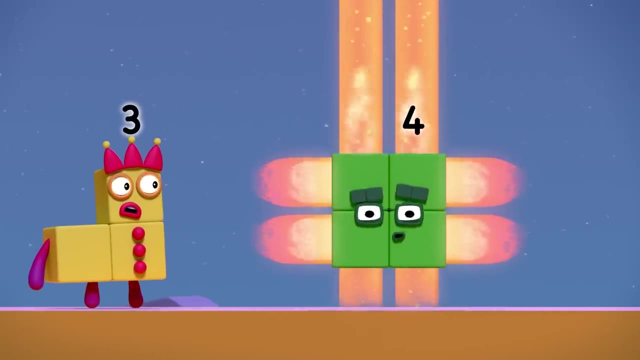 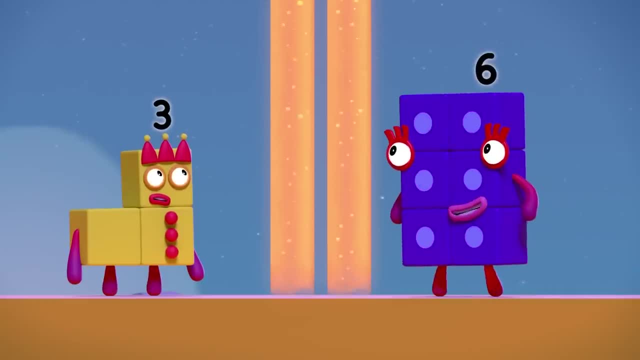 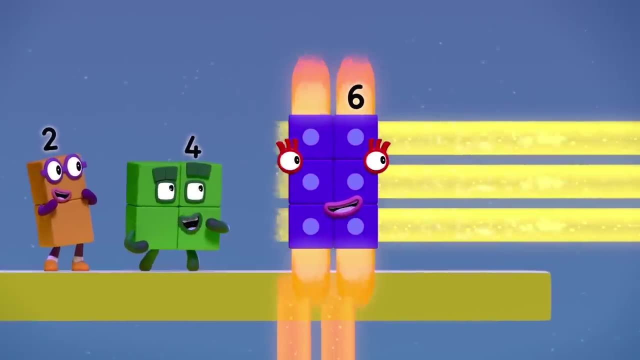 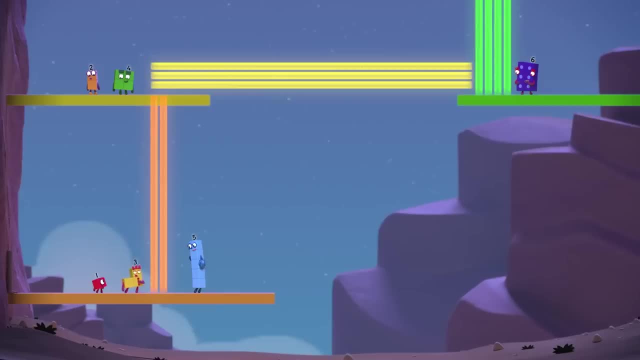 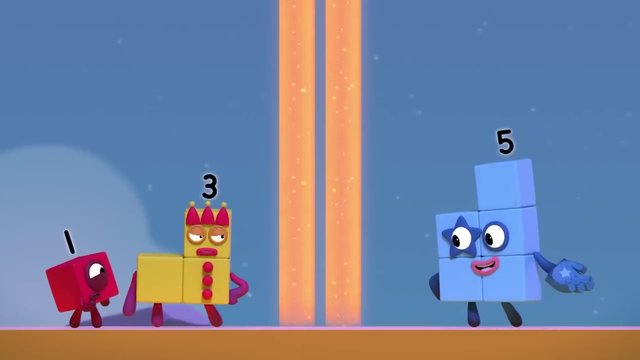 Woo, I'm two, lots of three. I've got two rays and three rays. I've got three rays too. you know, I could ride across just like Six if I could get up there. Odd numbers like us just can't make a rectangle. that's two blocks wide. 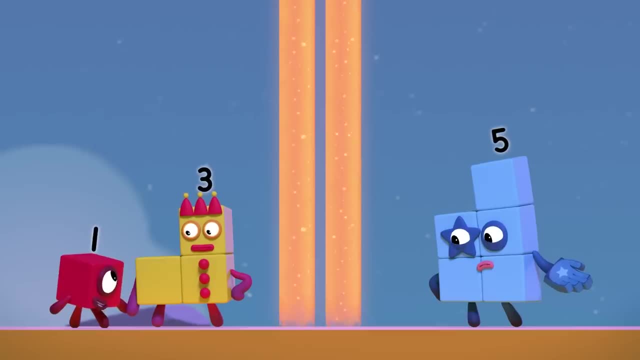 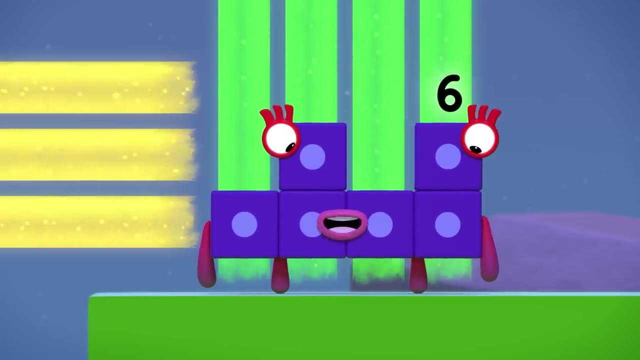 Twelve said only one of us had to get to the top. remember, We can all work together to find a way. I don't see how, I don't know. I don't know, I can't make four blocks. I'm a super-rectangle. 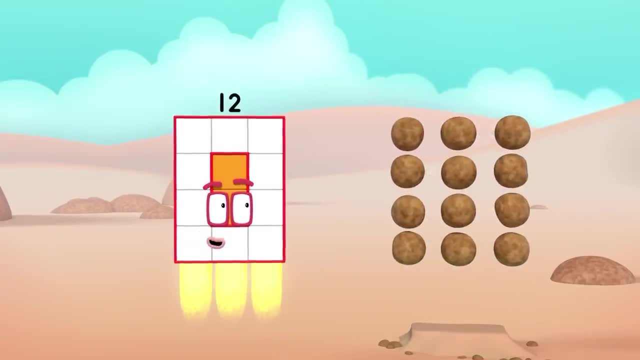 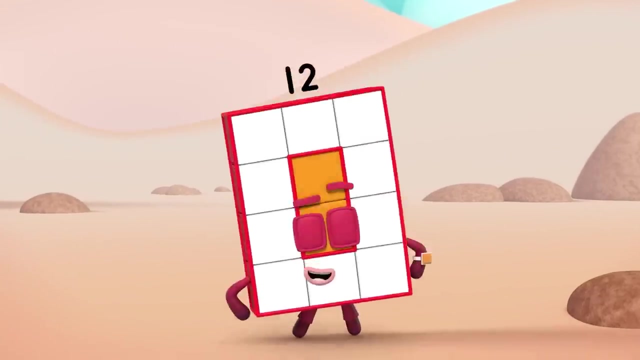 The rocks are in columns and rows, My blocks are in columns and rows And that's called an array- Array. Hey, I'm rectangular 12. I'm 10 and 2. I make arrays. that's what I do. 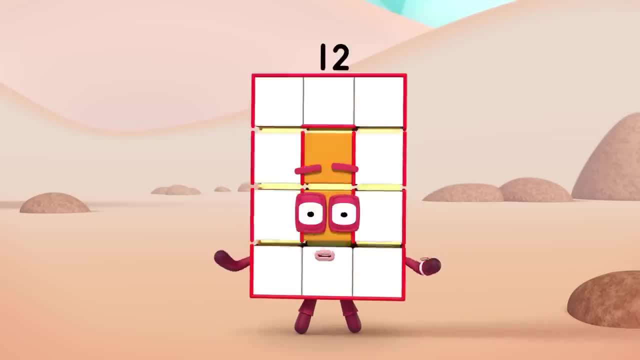 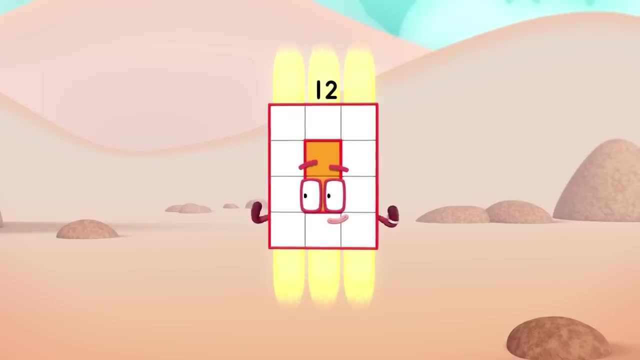 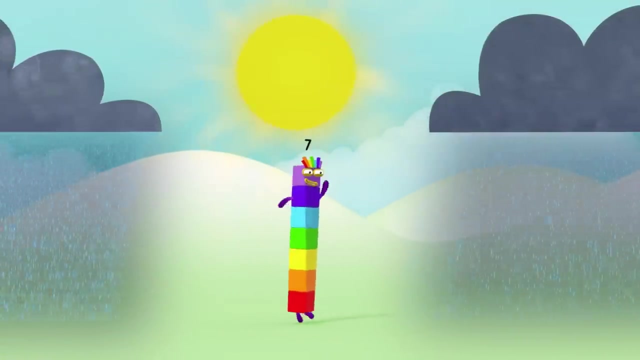 When I put my blocks in columns and rows, I make an array, and my rectangle goes like this: Three By four. Today's the day for an array display. I'm lucky number seven. I'm in a happy place, The sun is always shining and there's always 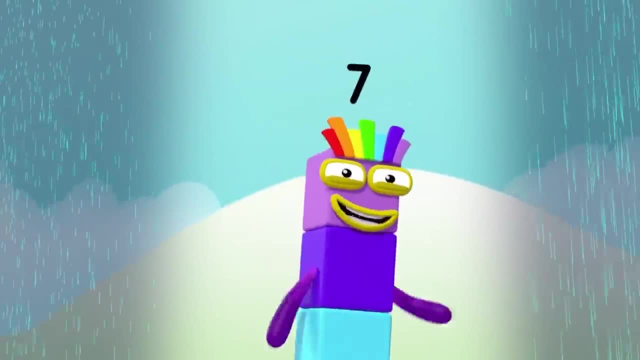 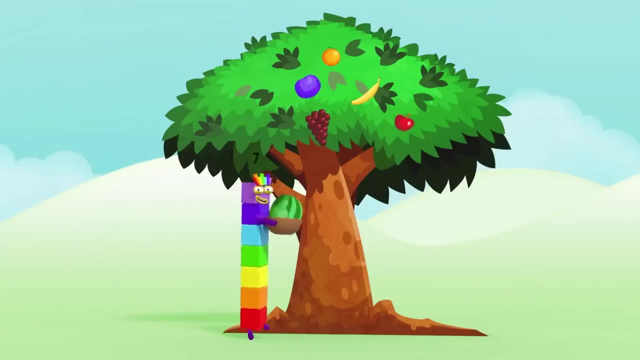 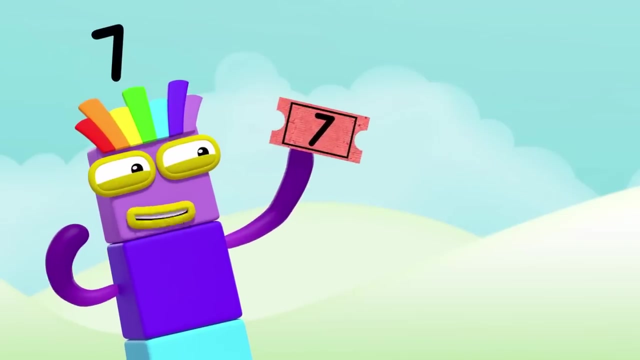 A smile upon my face. I see a penny and I pick it up And all day long I have good luck. I'm lucky number seven And everything is falling into place. I'm lucky number seven And, as you might have guessed, I always win the raffle. 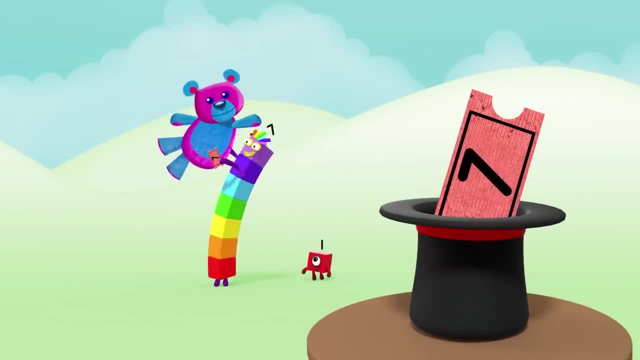 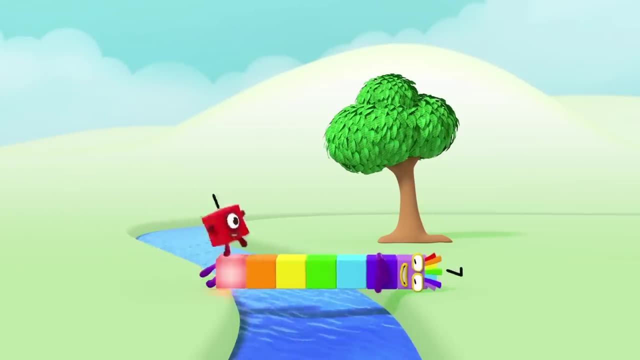 With seven on your side, you're seven less In a pickle. you're in luck. I'll help you out when you get stuck, And if you stick with seven, everything will work out. Everything will work out for the best, Yay.